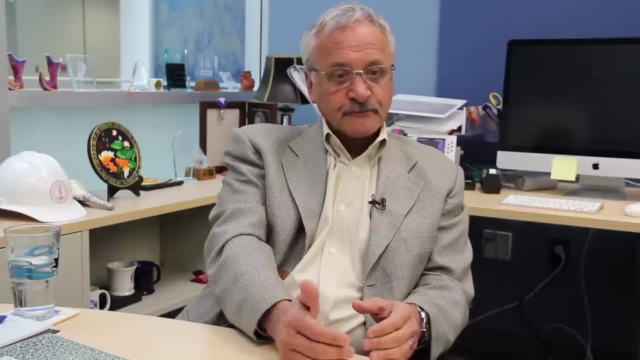 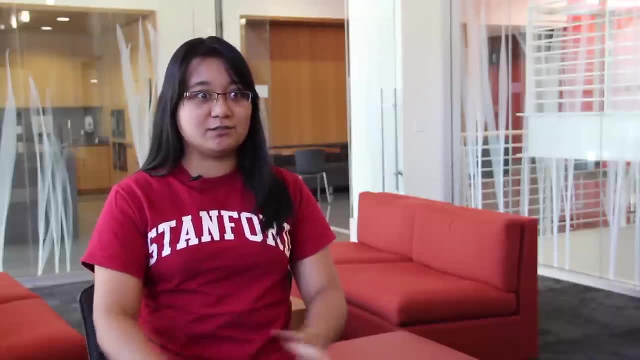 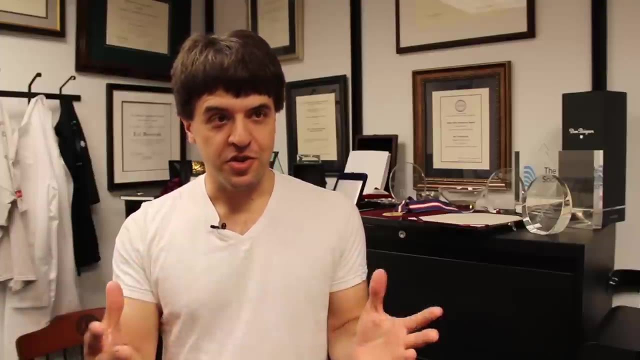 to have a fully approved undergraduate major. Bioengineering is really an interdisciplinary field, so you're not just taking a biology course and an engineering course and sort of calling it quits. Engineering is thinking about how a complex system works and making it work by understanding its components and how they work together. We go to our phone. 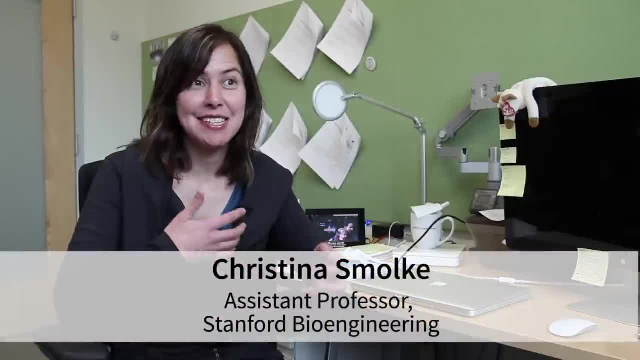 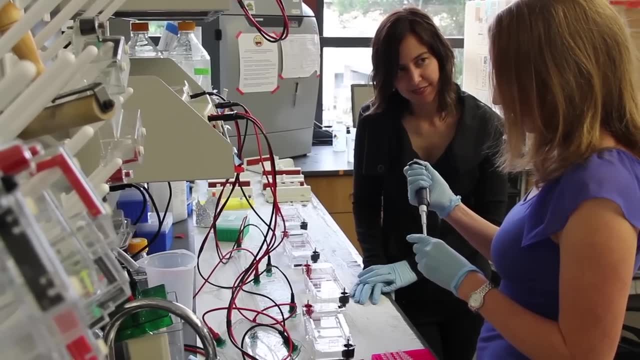 we expect it to be the same today as it is a week from now, as it is a month from now. That contrasts very sharply to biological systems, which are living systems. When we go in and engineer a biological system, we might engineer it for a particular type of behavior, but we have to as engineers. 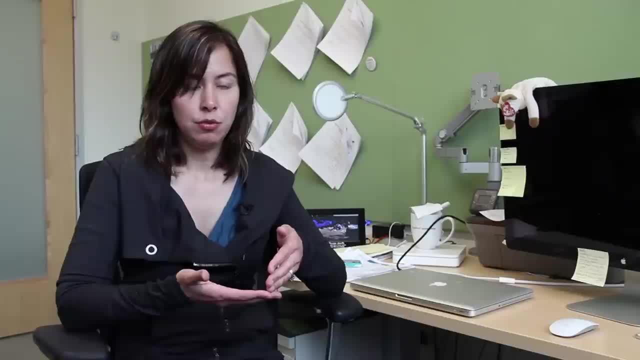 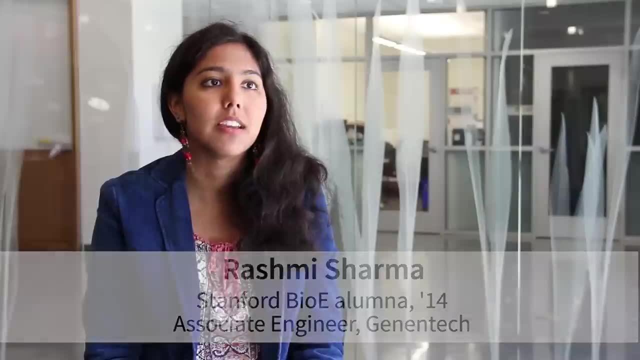 ask ourselves: what will that system be doing in a week from now or a month from now or a year from now? The thing that I think helps us get through the best through bioengineering is just the tight-knit community in the students and the TAs and the professors. For me it 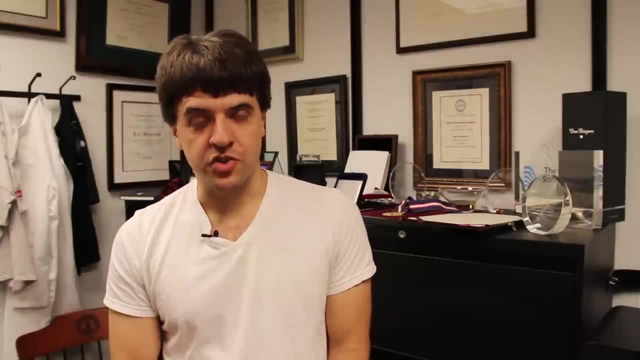 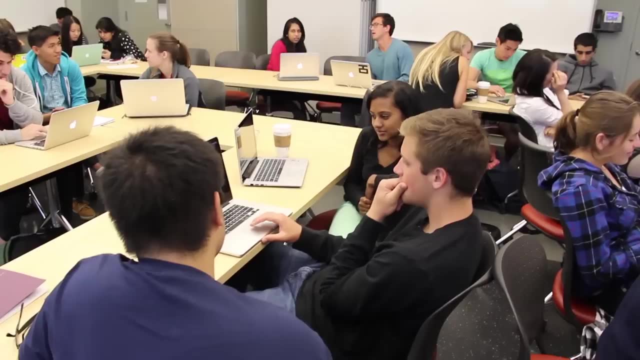 was one of the best things I ever did was to come to join the bioengineering department at Stanford, and it shaped my whole career in a very positive way. The opportunities that are created at the intersection of bioengineering and bioengineering, the opportunities that are 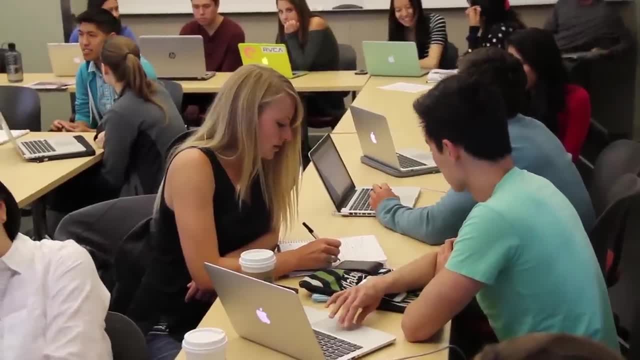 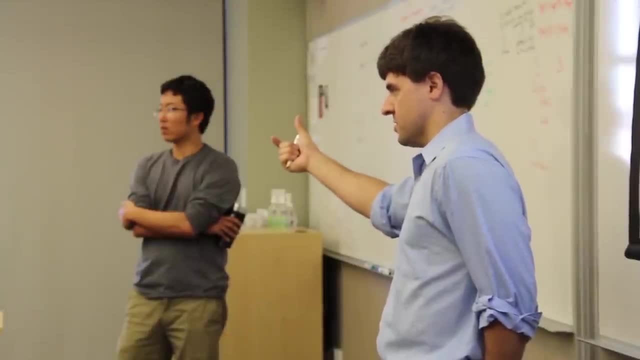 created at the interface of biology and engineering are immense and are only really beginning to be capitalized on, and I want to help create the same opportunity for the students, for undergraduate students at Stanford. The more mature we get, we get encumbered by our preconceived 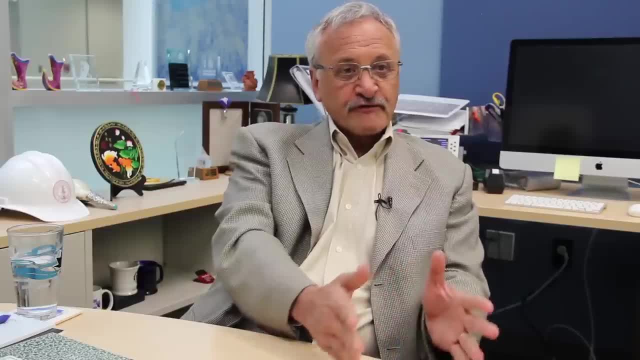 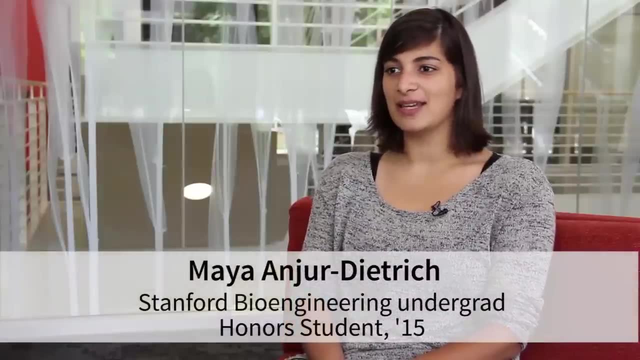 ideas of what's doable and not doable. Undergraduates are free from that. They don't know what they cannot do and therefore they're fearless. It's really exciting, because anything you want to do is probably the best thing you can do. 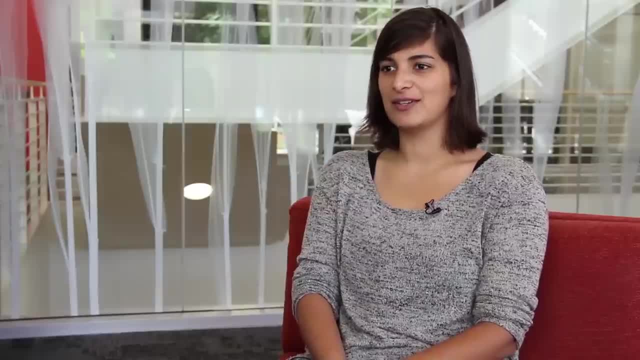 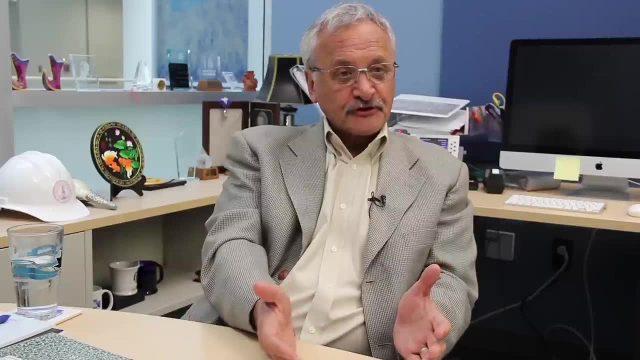 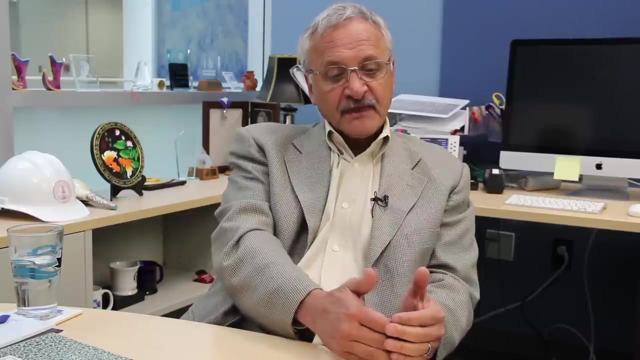 You can be part of bioengineering if you look hard enough, and so I don't think you should let yourself be limited by what other people have done, because maybe they just haven't thought of what you want to do yet. It is very meaningful to us and a great achievement, a milestone that the university now has endorsed. 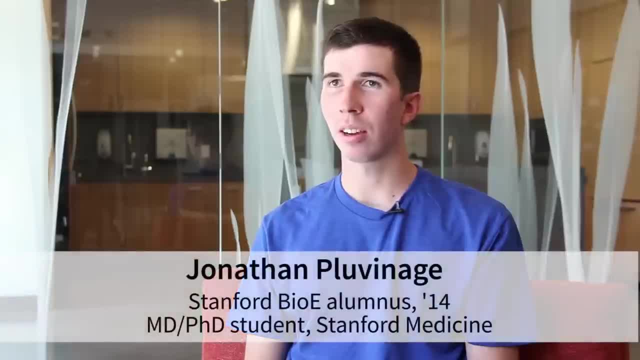 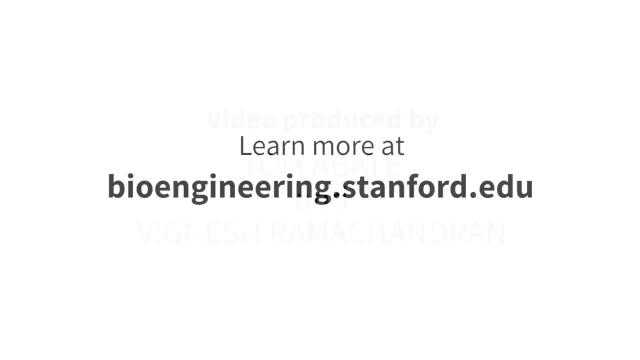